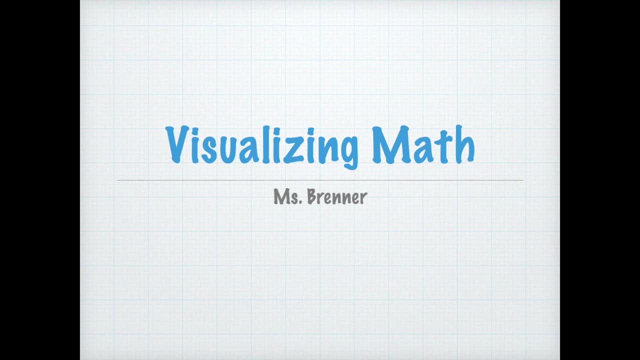 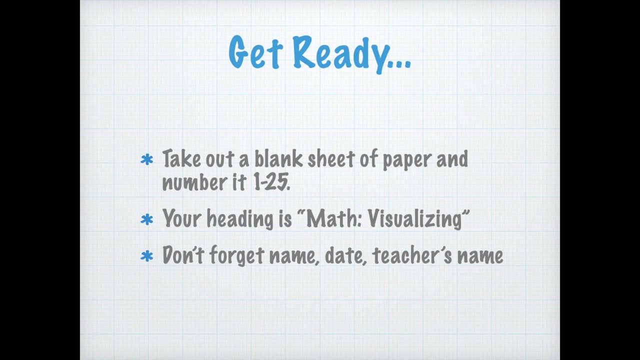 This is a very fun activity and a great way to get everybody started. It is called subitizing For those of you who are familiar with it, but I just like to call it visualizing math. Here is what you need: You need a blank sheet of paper and I need you to number it 1-25.. 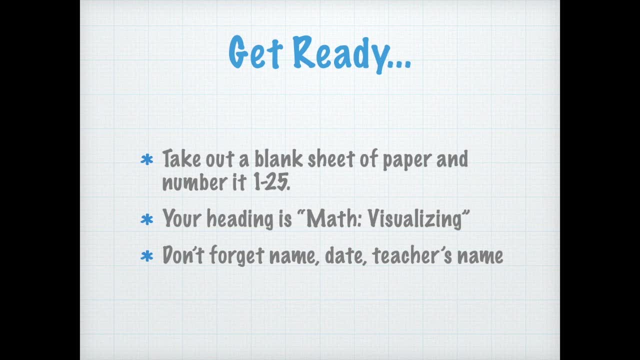 I'm going to be giving you some rapid fire questions. Just an image to look at and count how many is in the image, kind of thing. At the top of this paper write math colon visualizing and number it 1-25.. If we were in the actual classroom I'd make you put your name date. 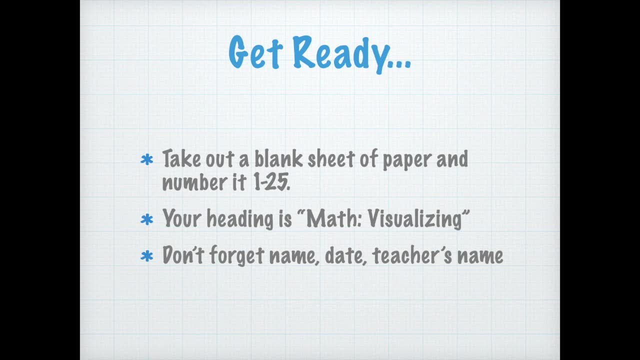 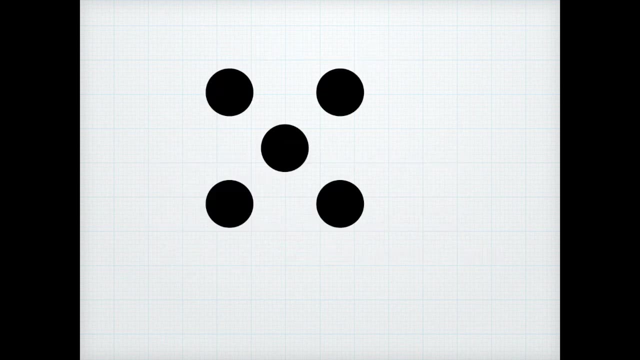 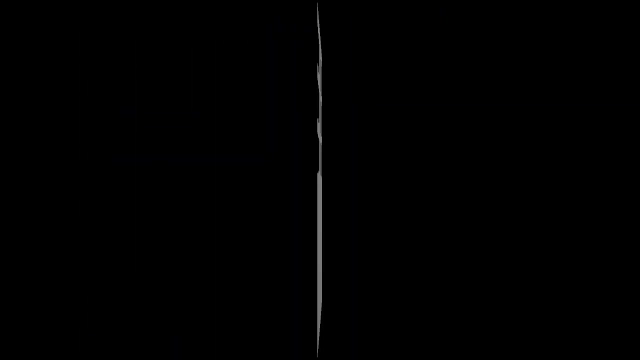 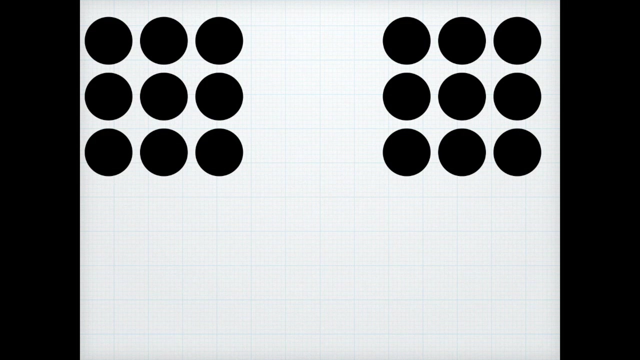 and teacher's name, but you're at home so you can skip that part. Pause the video if you need more time. Number one: write how many you see here. You should have written the number five. Number one: five. Here's number two: Write down how many you see. 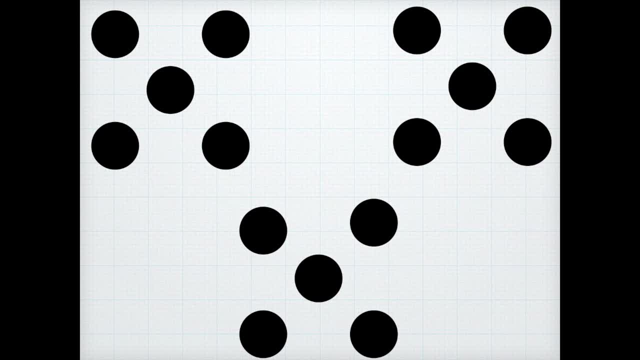 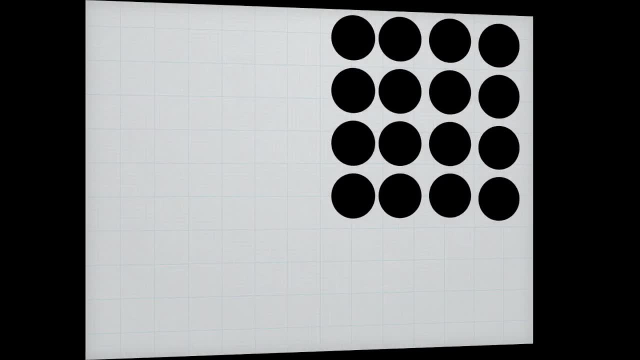 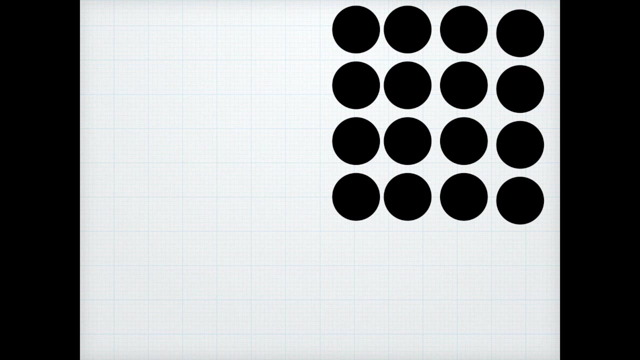 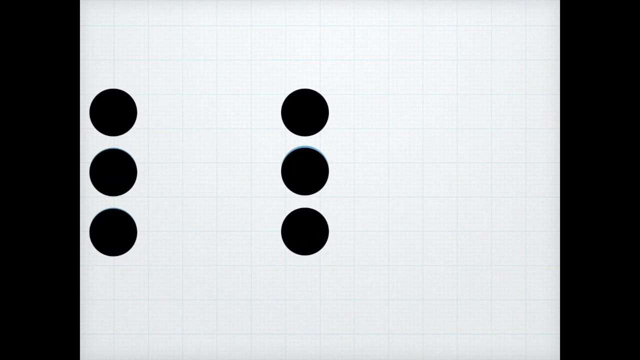 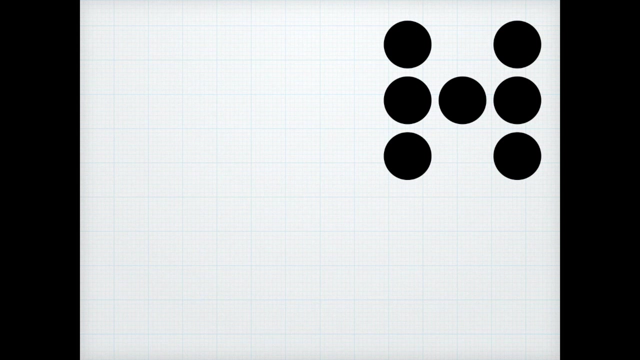 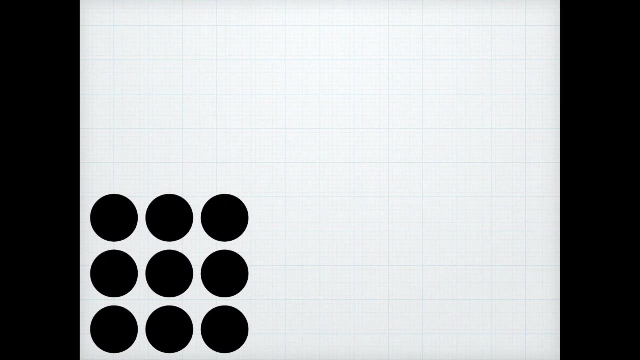 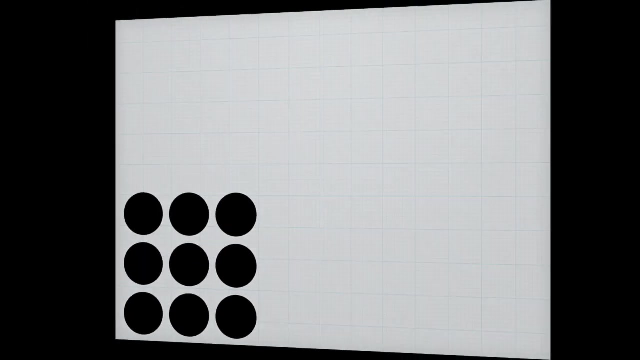 Here's number three. Time's almost up. Number four, Go ahead and do it. Number five: Here's number six. Number seven. Here's number eight. Number nine. Here's number ten. Here's number eleven. Here's number twelve. 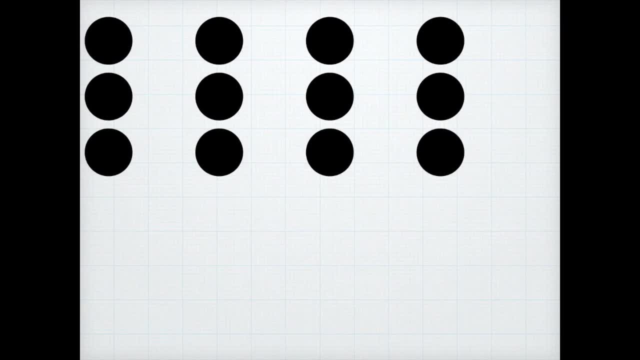 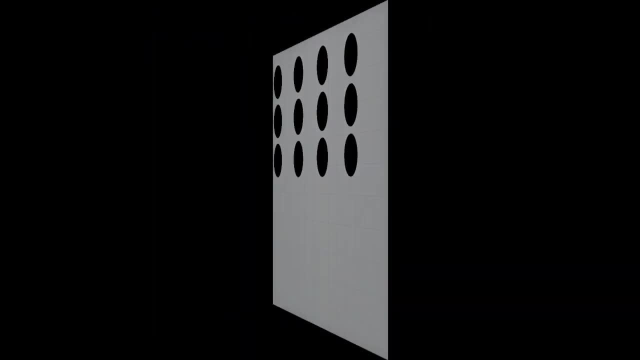 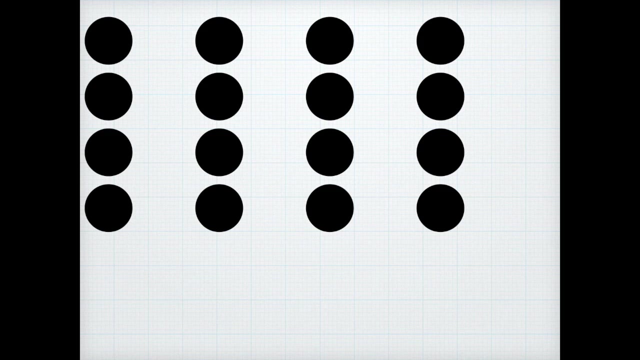 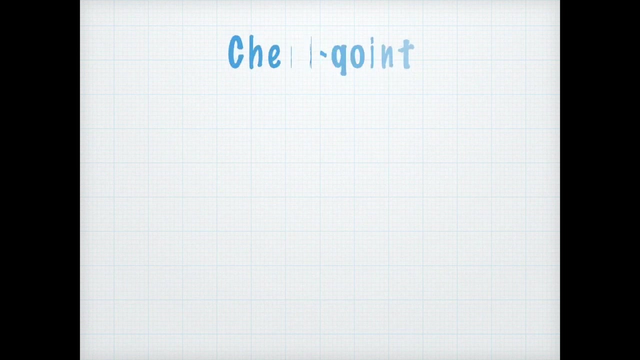 Here's number thirteen. Here's number fourteen, Number twenty, Number twenty. Here's number thirty, Number twenty, Number twenty, Number twenty. All right, Alright, so here comes our checkpoint. You should have finished number 1-10,. and if 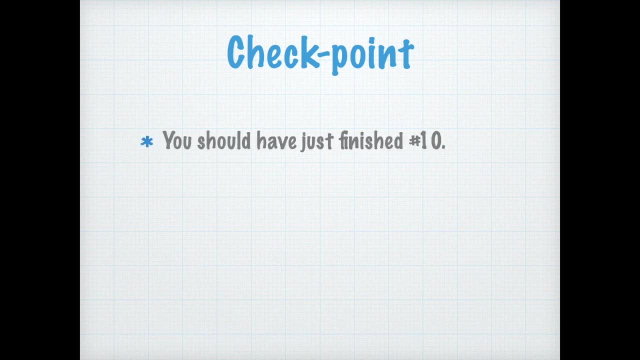 you didn't do that, don't worry, Just start on number eleven. Okay, So here comes number 11.. Now they are going to go a little bit faster, So get ready, get set. here's number 11.. Big deep breath. 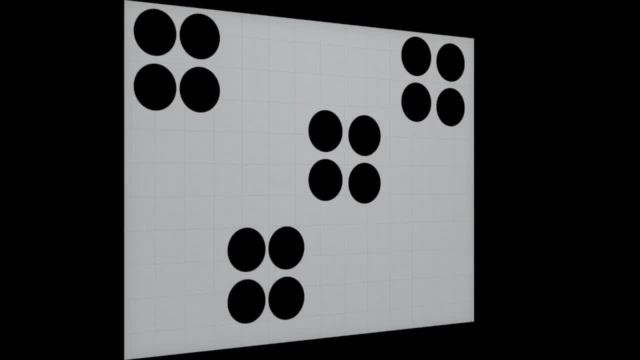 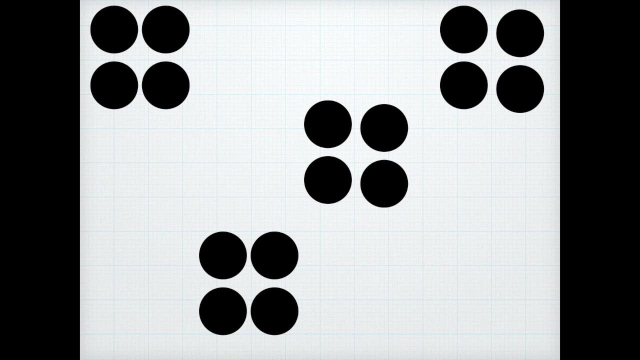 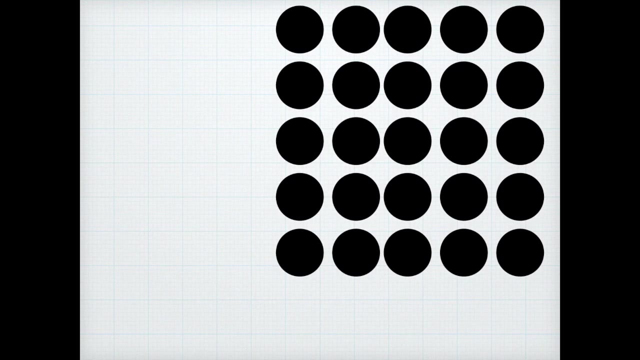 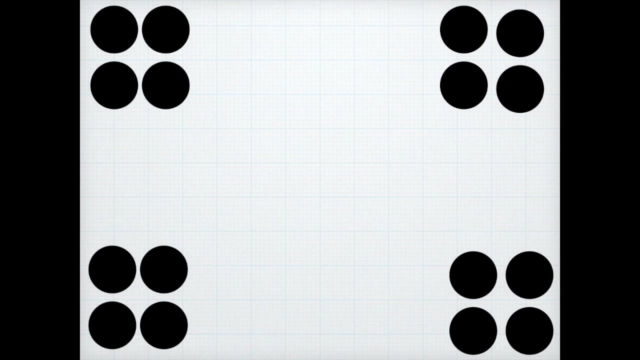 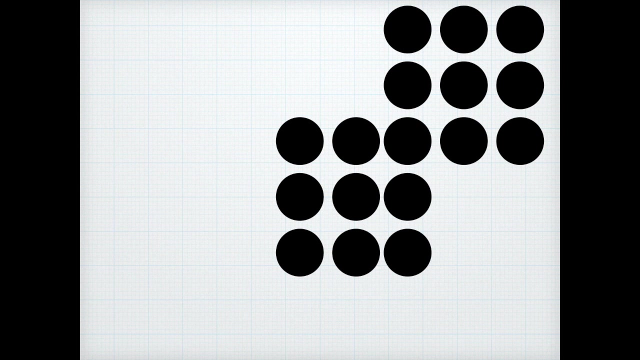 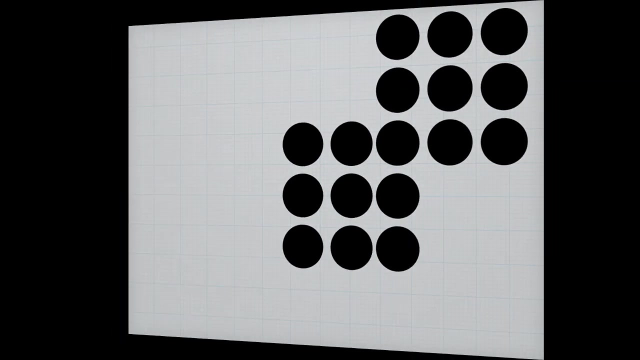 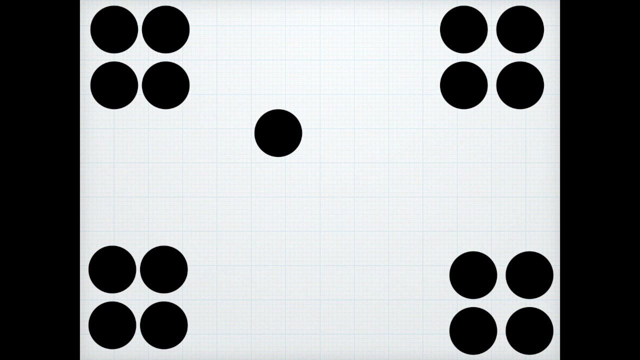 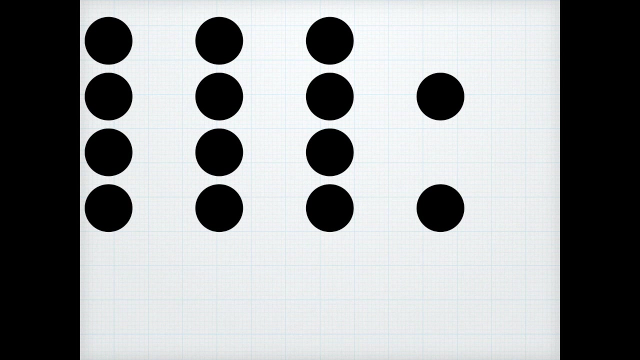 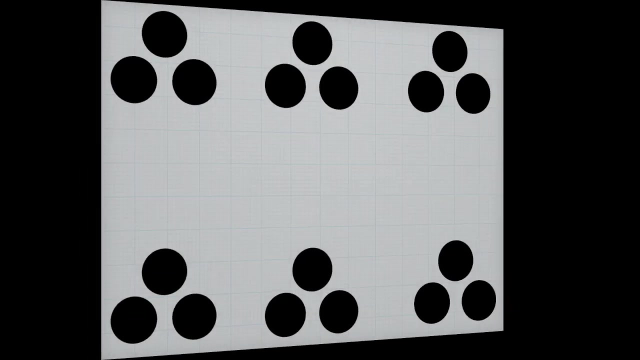 Number 12.. Okay, don't start counting all over again. Use a strategy to figure out how many is here based on the last problem: Number 13.. Number 14.. Number 15.. Number 16.. Number 17.. Number 18.. 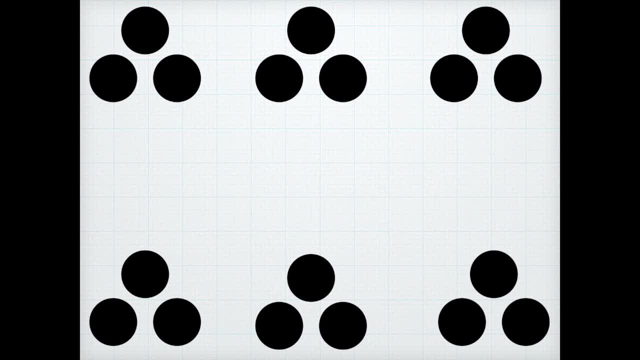 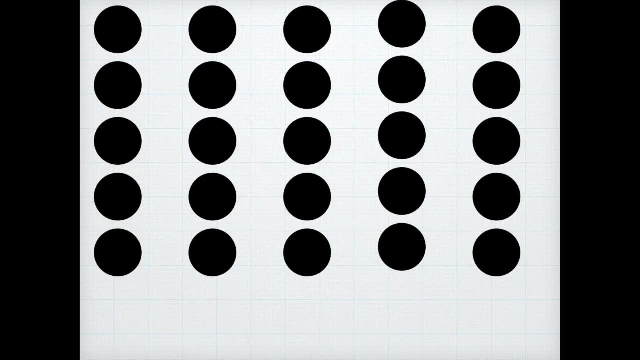 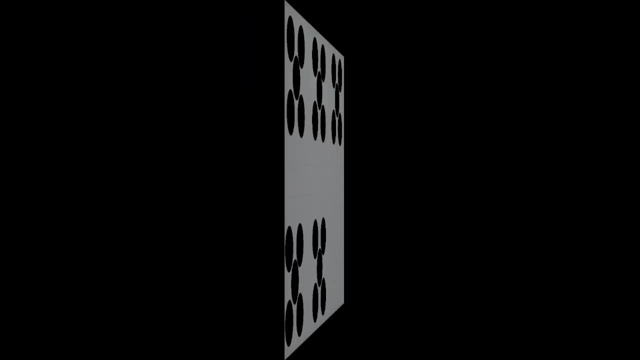 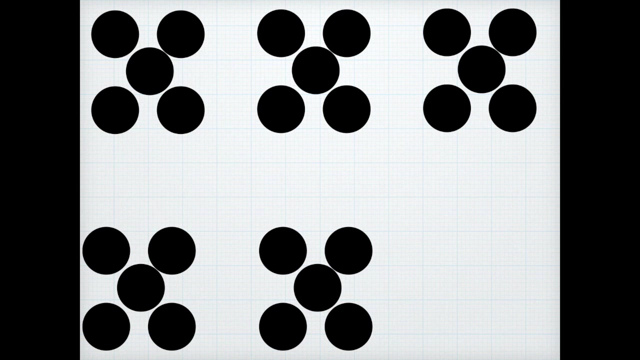 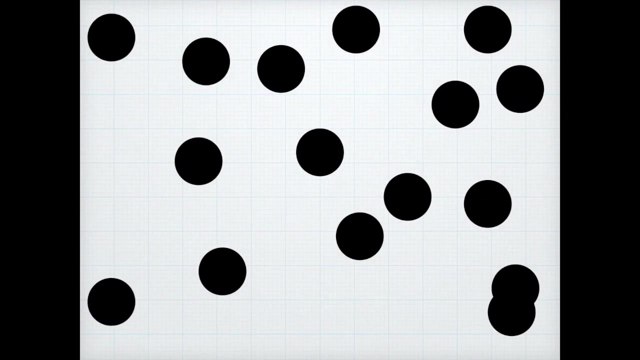 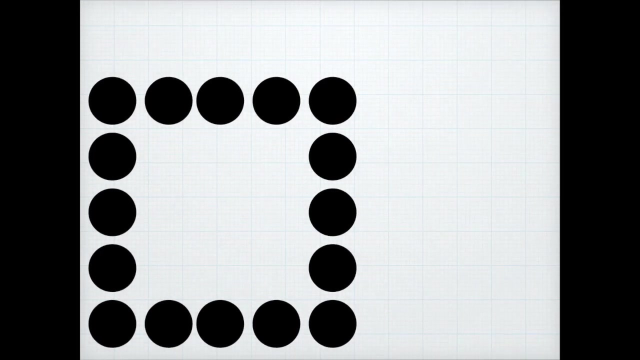 Number 19.. Number 20.. Number 21.. Number 22.. Number 23.. Sorry, I have to laugh because this one you have no strategy Right. This one you literally have to count one by one, Sorry. Okay, back to strategies. 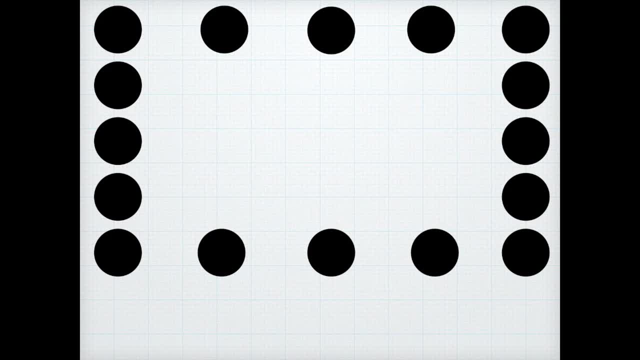 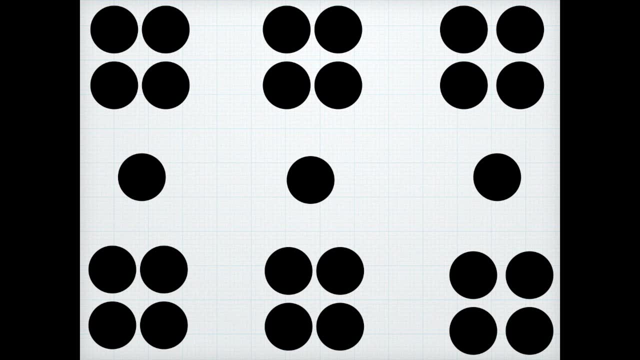 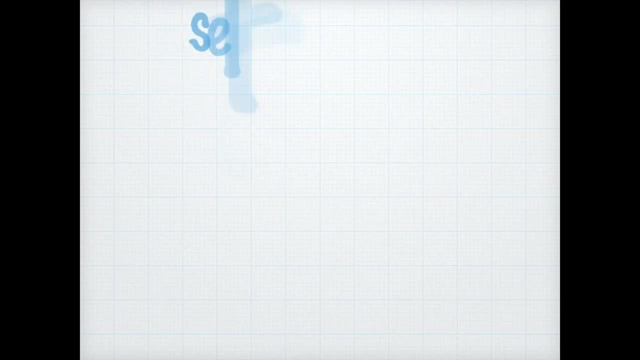 Okay, so now you should have gotten all the way to 25.. And we'll be talking about in groups how you viewed each one, So let's take a quick look. The answer to number one is Aw, I'm not going to tell you.